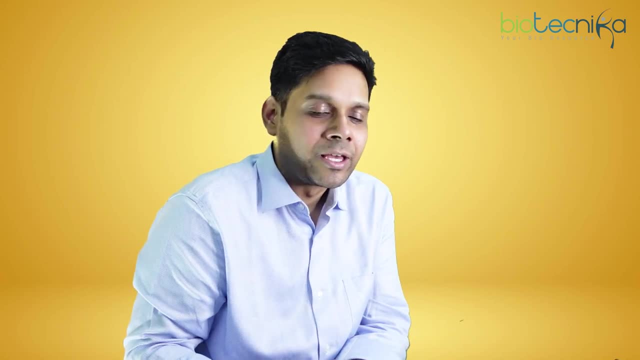 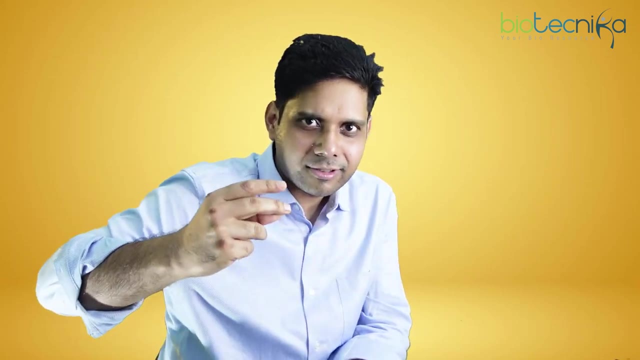 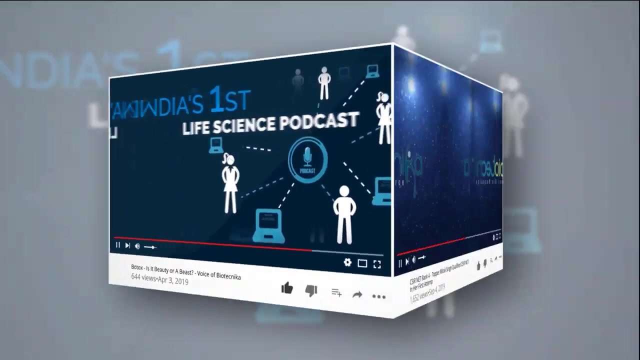 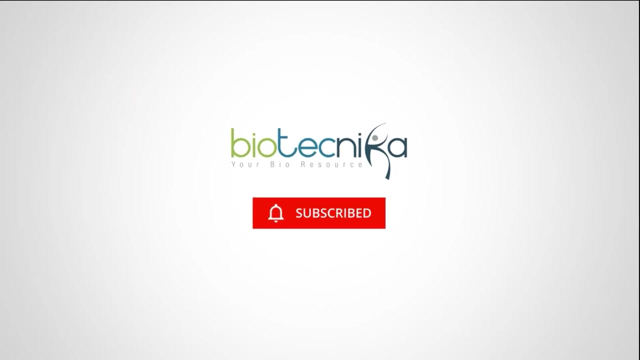 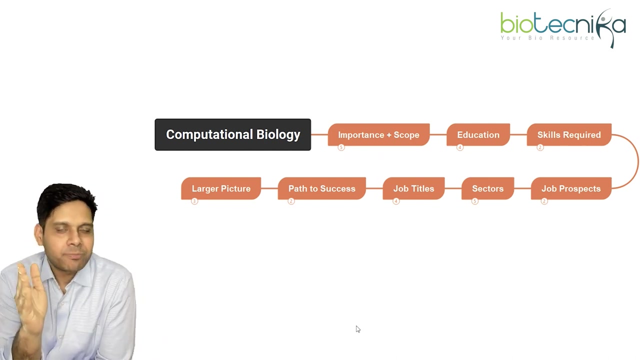 next time when you jump in, you know where you are sailing. So let's get started with today's video. So today we are talking about computational biology. as you can see at my back. We'll start with the first part, which is importance and scope. Okay, let's look at. 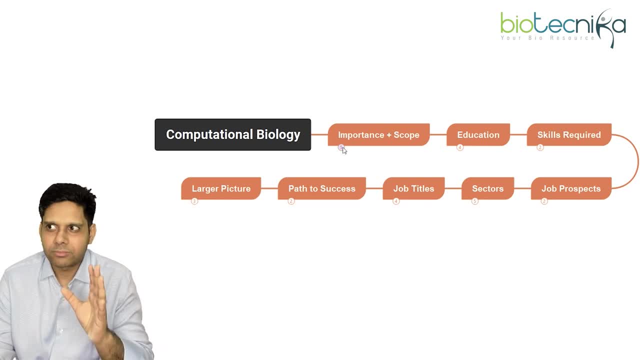 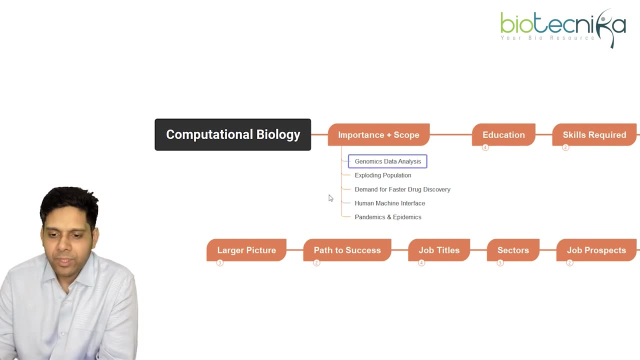 how important this field is. Well, we know how the IT revolution happened in India and in the global arena, but how it can help us in the biosciences industry. Well, with the advent of technology, we have more and more genomics data which is being available today. So analysis of 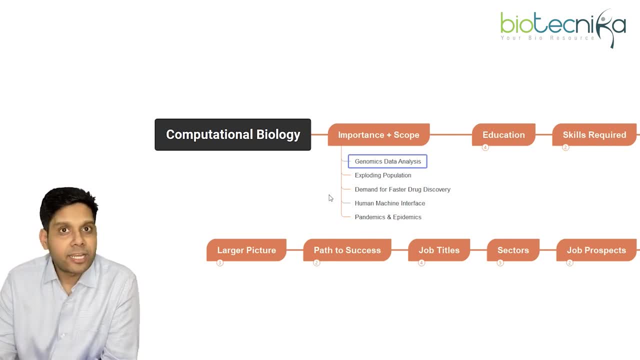 that banta hai. So that's one thing. genomics data analysis is one area which is very scoping and growing. The population is exploding at the moment. The population is exploding at the moment. The population is exploding. that means newer avenues of application of computers in biology is coming. 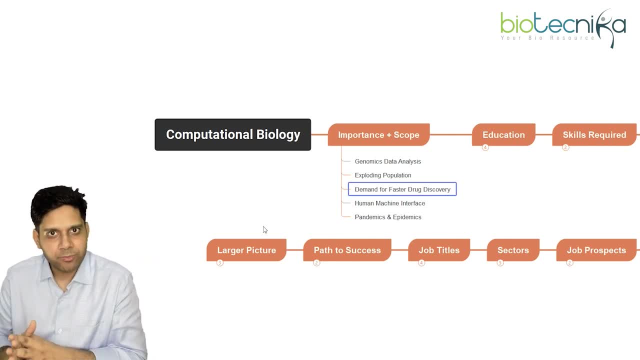 upThere's a huge demand for faster drug discovery process because the microbes are getting smarter and outsp variating humans. so we have to take help of computers to, you know, develop better drugs, faster drugs with much more efficacy. Next, human machine interface. you must have heard of ellen mask. 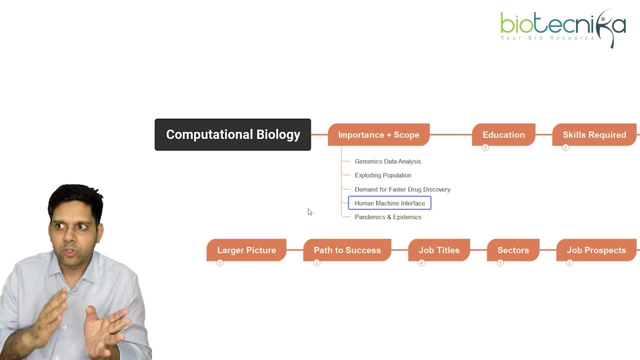 and the brain machine interface which they're developing. Tomorrow, what if I tell you that this is going to be the new normal? So for that, more and more computational biologists, neurologists, are required. And the last one: pandemics and epidemics Everywhere, everywhere you're seeing. 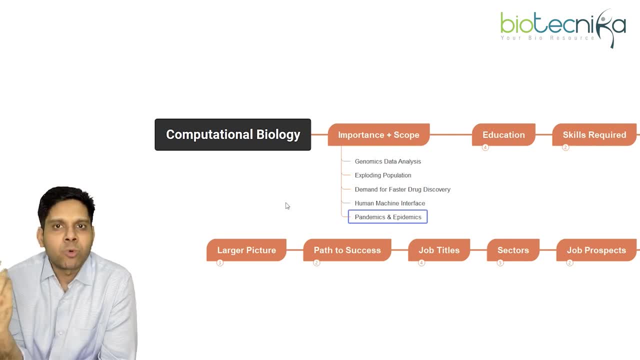 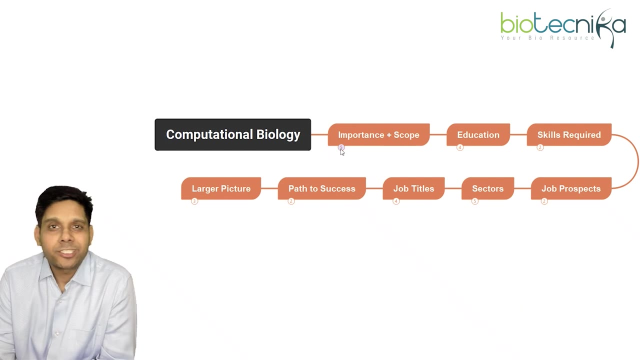 pandemics, epidemics happening, and that demands for more application of computers in biology. In fact, the Moderna RNA vaccine was designed inside a computer and not in a lab, So isn't that amazing. These are the pointers which definitely highlight how important and scopic 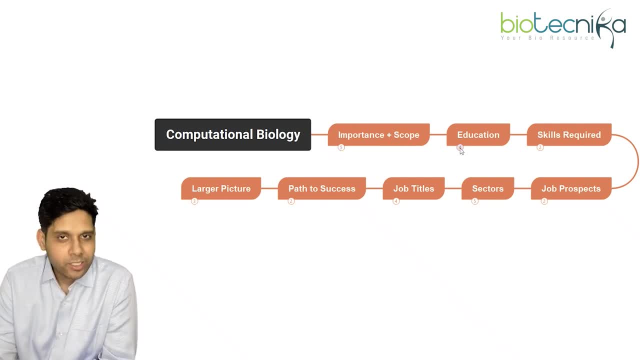 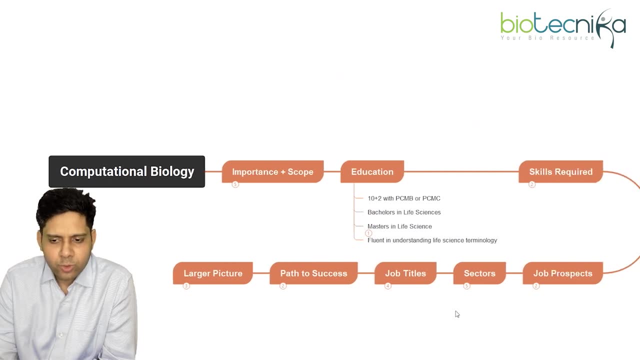 this field is going to be in the future. So what are the educational requirements you need to get into this field? Well, it's very basic. You should have a 10 plus 2 with physics, chemistry, maths, biology or physics, chemistry, maths, computers. You should have a bachelor's in life. 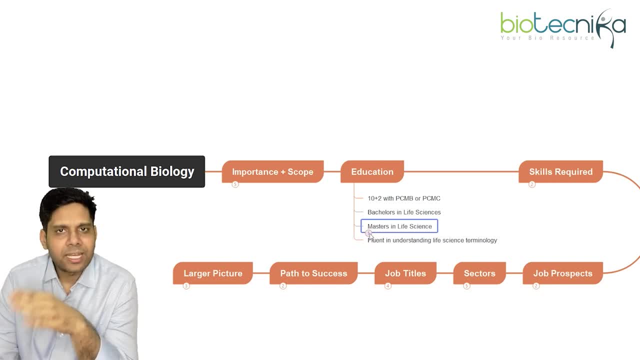 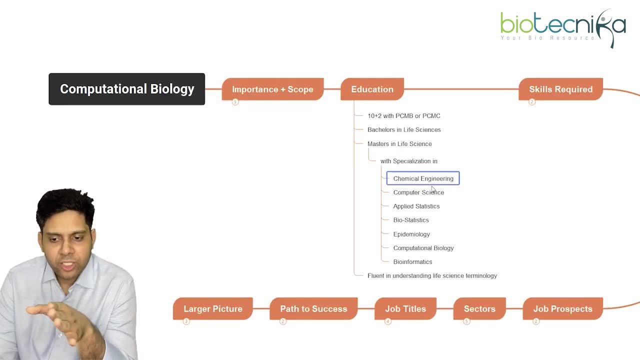 sciences And while you're doing master's in life sciences, you can take up special specialization. And what are those specialization Any of these you can take? You can take a specialization in chemical engineering, computer science, applied statistics, biostatistics. 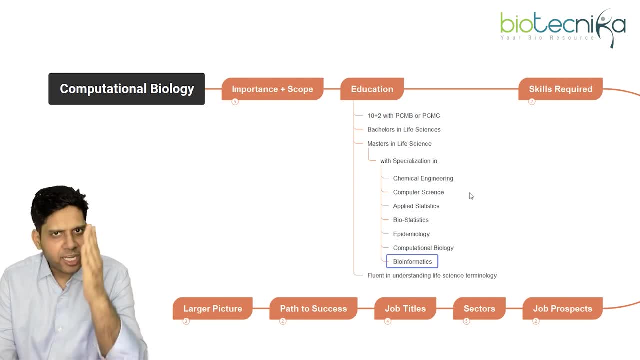 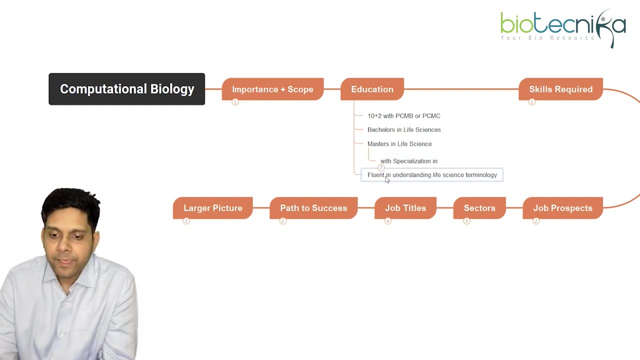 epidemiology, computational biology and bioinformatics. Any of these you can choose as per your interest, And that will further help you excel in this field. The next one: you should have a fluent and very good understanding of scientific terminologies: biological terminologies, biochemistry, molecular biology, genetics. 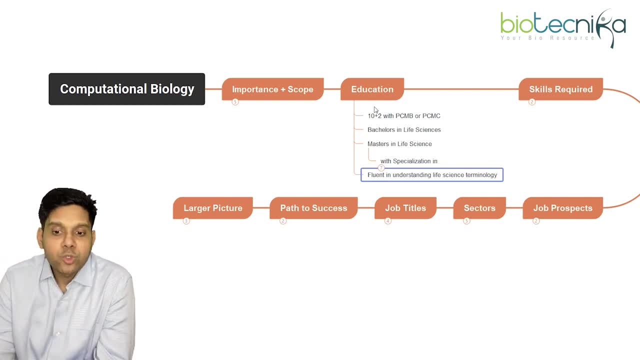 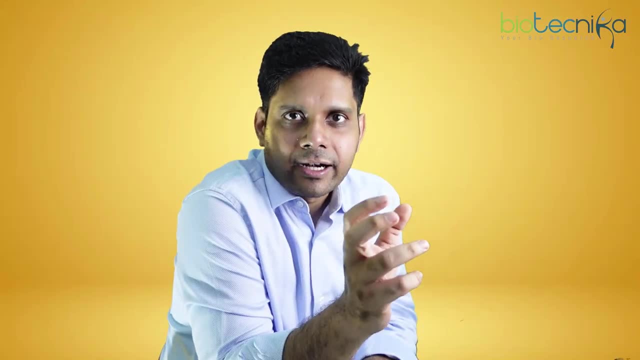 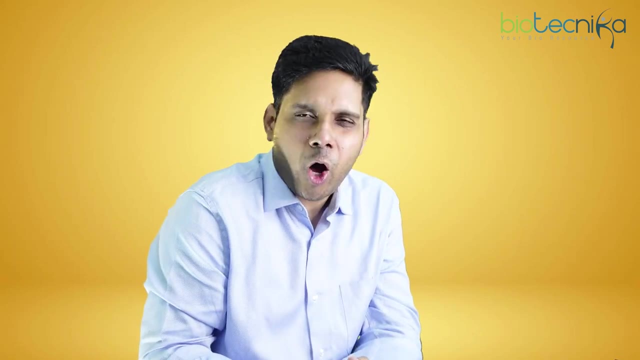 all this you should be thorough with. So these are the educational requirement. But hey, is this enough? No, You see, this is an upcoming field. That means things change overnight. New softwares are coming, new ways of doing things are coming, And that means you need a lot of skill set. 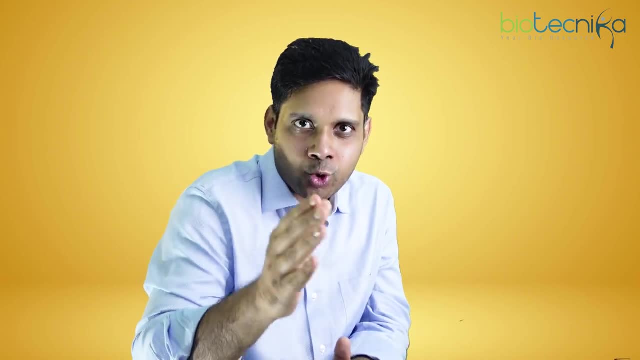 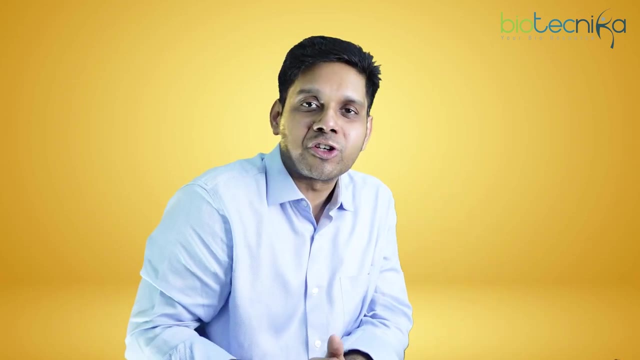 So I am going to classify the skill sets now and show you- and probably during your bachelor's itself, from bachelor's or master's, whenever you are, and wherever you are, you can start building on the top of your skill set. So let's get started with the skills required. So I'll divide it into two parts. 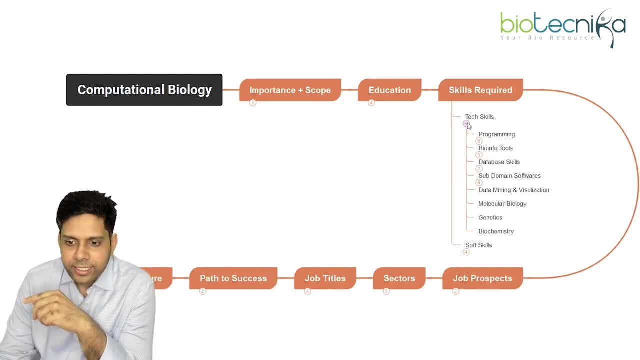 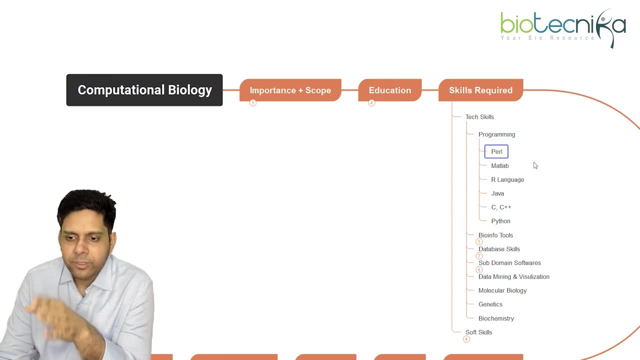 technical skills and soft skills. Okay, so the technical skills which you require is programming. So, under programming, you have- you have a lot of you know- languages like Perl, MATLAB, R language, Java, C, C++, Python. all this you should know. Next is bioinformatics tools like cluster law. 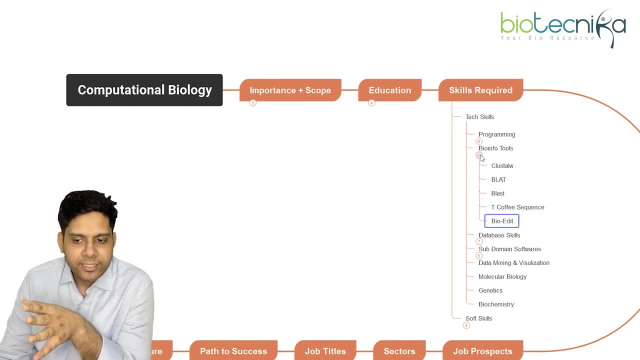 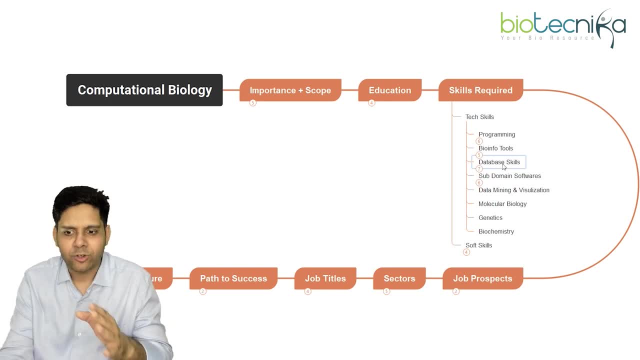 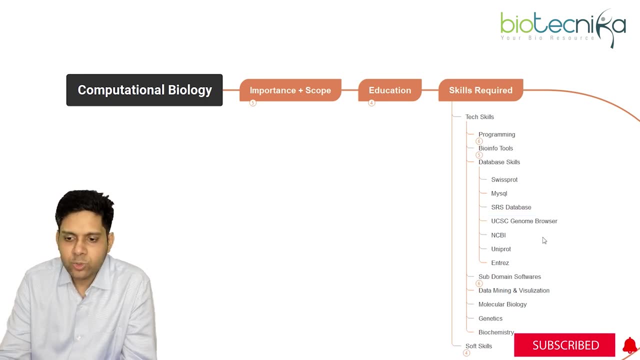 These you have to study over a period of like 10 years, right? So it's not that you're going to do it overnight. Next, database skills like SwissProt, MySQL, SRS database, UCM, SC, Genome Browser, NCBI. 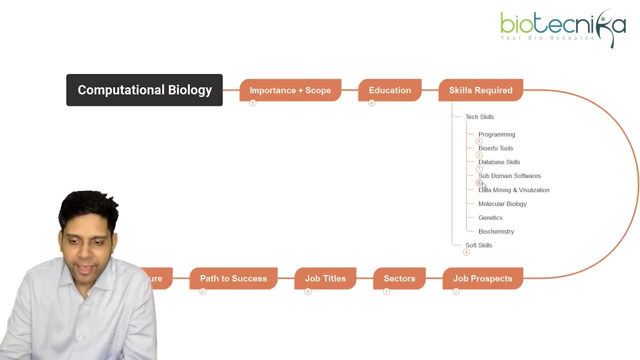 Uniprot, IntraS. So these are the database skills you should have. Then subdomain softwares like OE, CHEM, SwissDoc, Oracle, Autodoc, Protmax, Argus. You see, these softwares are required because you are going to study the behavior of 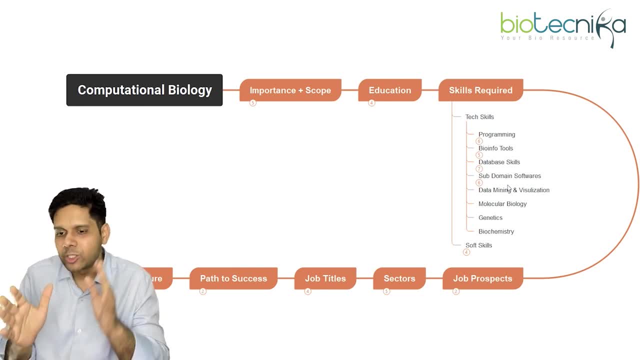 biological molecules at the physics level, at the atomic level. So you know these softwares will be very handy: Data mining and visualization, molecular biology, genetics, biochemistry. So these are the technical skills you require over a period of next five to seven years. 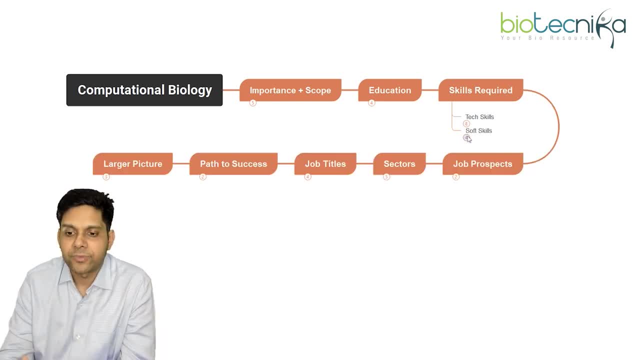 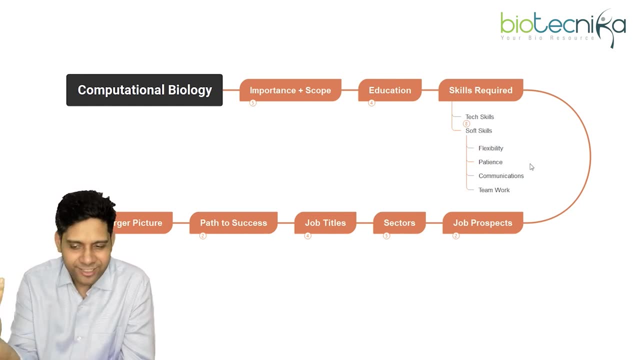 You need to develop this and that's where you can get into this field. Now, what are the soft skills required? Very simple: You have to be flexible. You have to have a lot of patience, because obviously, research requires a lot of patience. 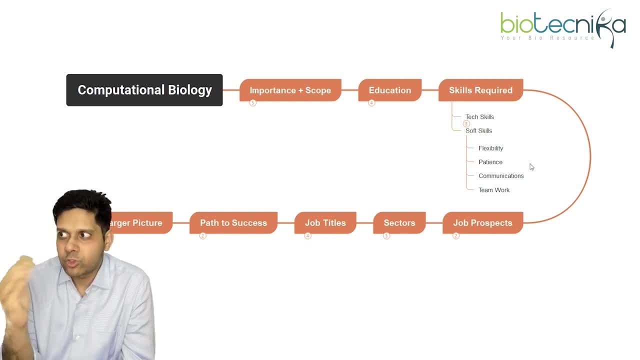 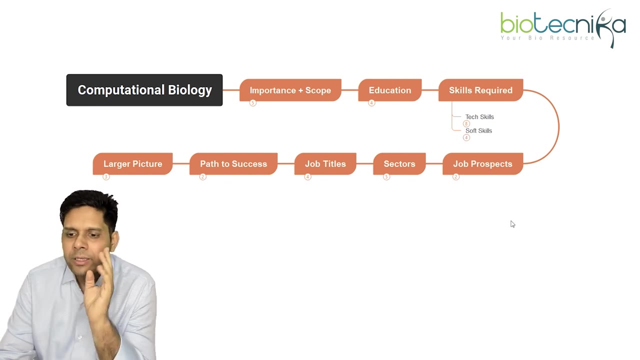 Communication. you need to be very clear with what you want to communicate with your seniors, superiors, peers and juniors. and teamwork, because nobody in this world can move one step forward without teamwork. OK, so teamwork is a must. So these are the soft skills. Of course, there are a lot of soft skills out there. 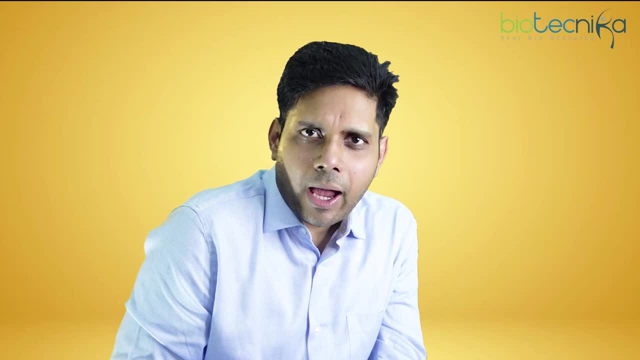 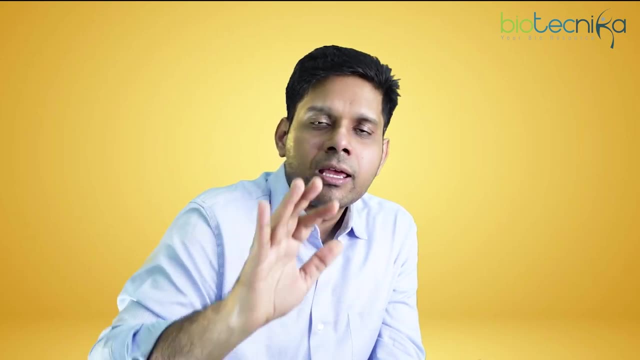 So now, quickly coming to the job prospects, Here is something I wanted to highlight. See, there are jobs in the government, there are jobs in the academics and there are jobs in the industry, But you need to choose, depending on what kind of life you want. 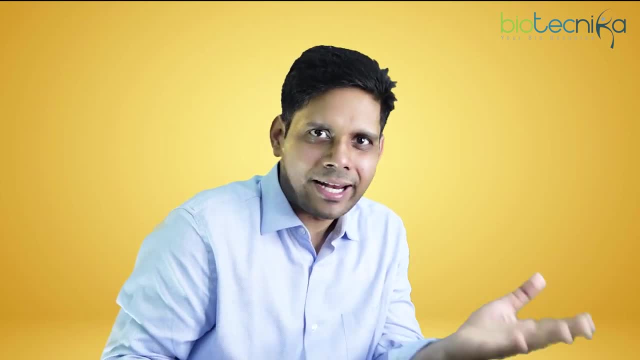 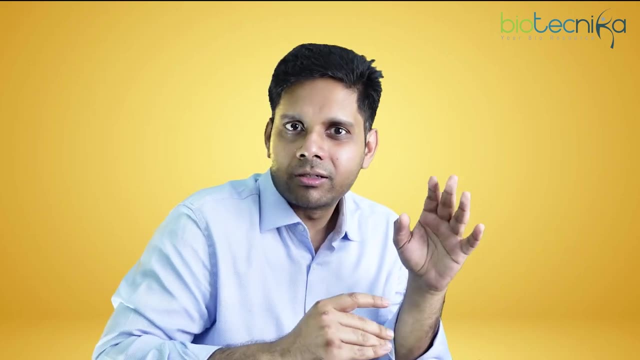 OK, Not the money side, because money eventually will flow and get spent. What kind of life you want? You want a stable, calm life. Get into academics. You want something like dynamic. too much of work? OK, workaholic. You're passionate about the field? Go for the industry. 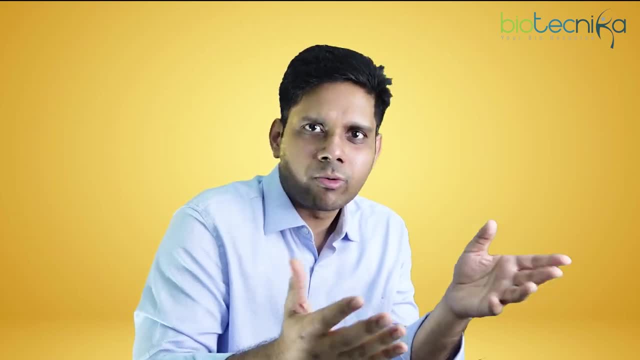 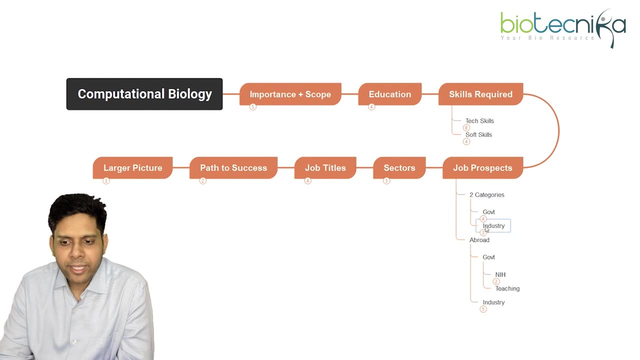 And if you're someone who just wants a stable government job, of course go for the government jobs. So that's where let's jump in. now to the job prospects. So job prospects, I am dividing into two categories: government and industry. 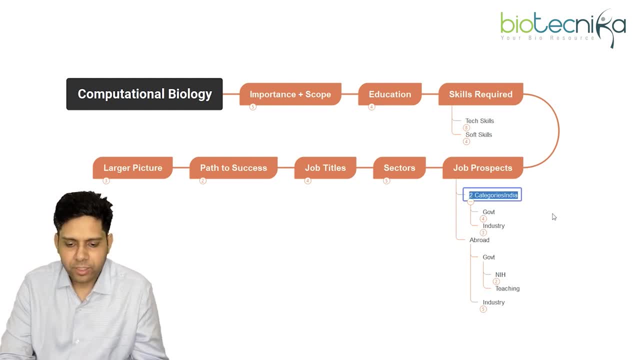 So here this is for India, So this is for India. So under government you have a lot of research happening or CSIR, in medicine, epidemiology, genomics And these CSIR labs. these are happening. And in academy also you can get: once you have CSI net qualified, you can get into as computational biology professor, assistant professor. 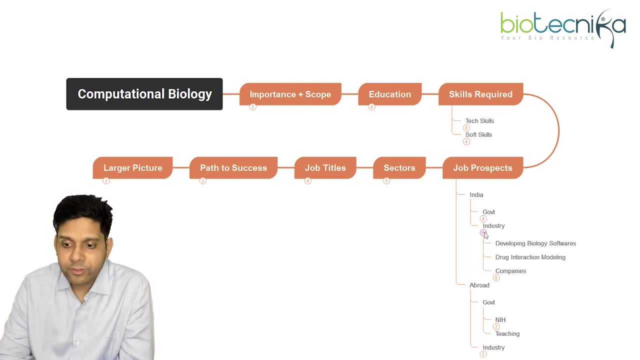 All that is there. Now, coming to the industry in India, you have companies which are developing biological software. You can get in there a software engineer, or you can jump into drug interaction modeling and uh doing using the softwares which i just showed you. now, what are the companies in india working on this? so you have 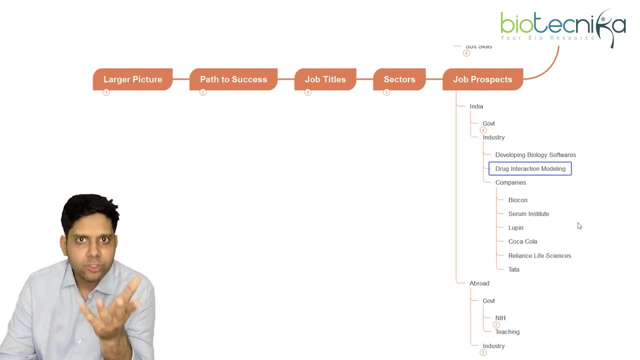 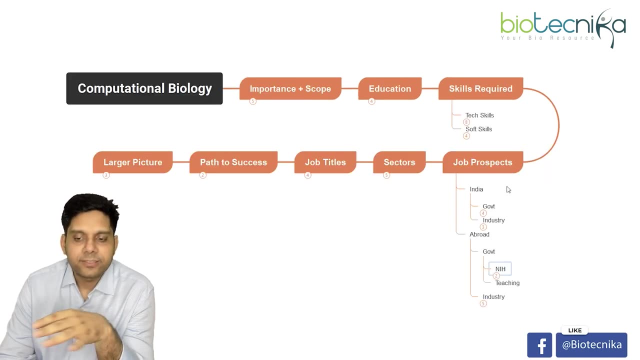 biocon serum issued lupin. uh, coca-cola scrotinger is also there, reliance life sciences, tata. so all these companies are working in this domain now coming to abroad. so let's look at: okay, there also we can divide into government and industry. so under government you have nih national institute. 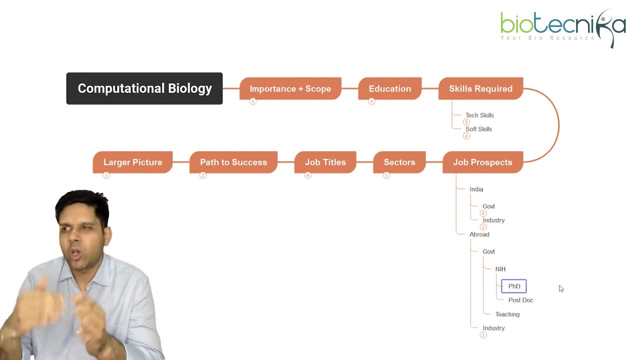 of health in us and they have phd and postdocs doing research, so you can get in there and do your phd or postdoc and, of course, multiple other positions are available in us for this. okay, and like i have always said, said, my us is the mecca of uh biosciences, so that's where you can get in. 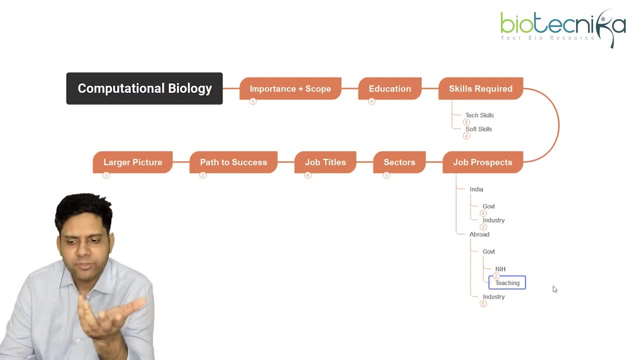 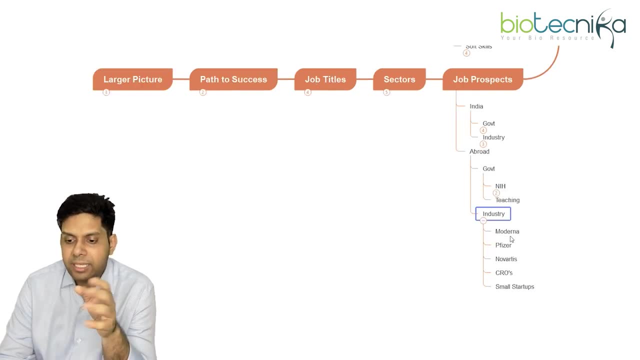 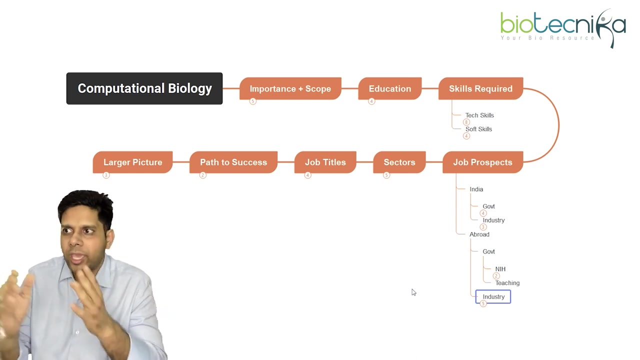 now teaching jobs also. you have teaching jobs- professor, assistant professor jobs- there in us and abroad. so now coming to the industry there. so you have companies like moderna, pfizer, novartis, various cro's and small startups working in this domain in the us, uk, europe, china. so you can. 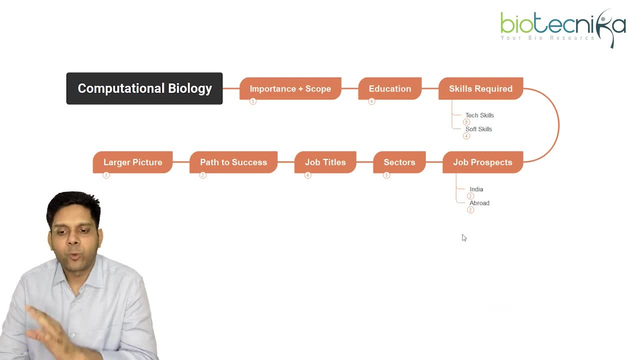 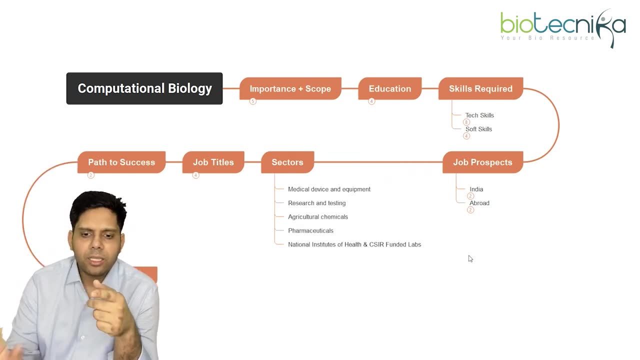 always get in there. now, very interesting thing here is: i'm going to now divide it into sectors, like: okay, i told you about indiana abroad, now what are the sectors you can get in? so you know, medical device, biomedical devices, research and testing, agricultural chemicals, pharmaceuticals, big pharma and various funded labs of csir and national institute of health that 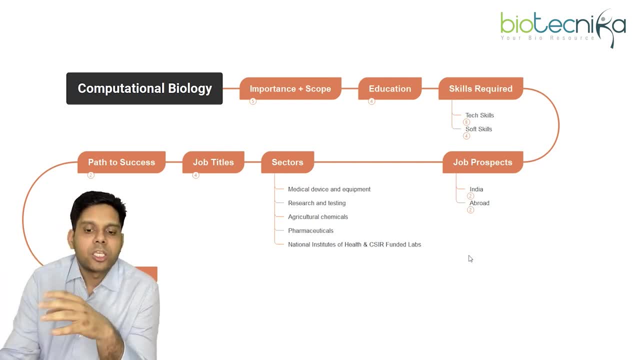 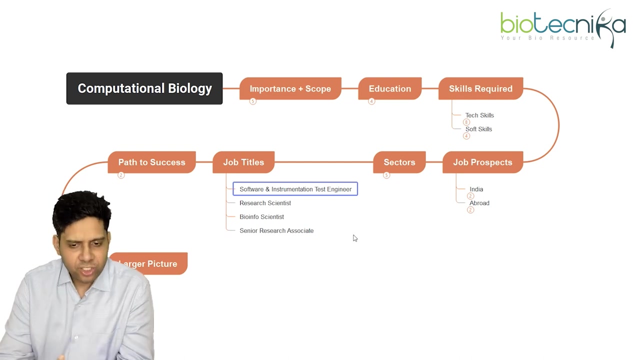 is nih in us, so these are the places where you can get in easily with a computational biology. but what kind of job titles you will get? okay, here it is so once you get in there, you will get a job title like a software and instrumentation test engineer. you may get a job with a title. 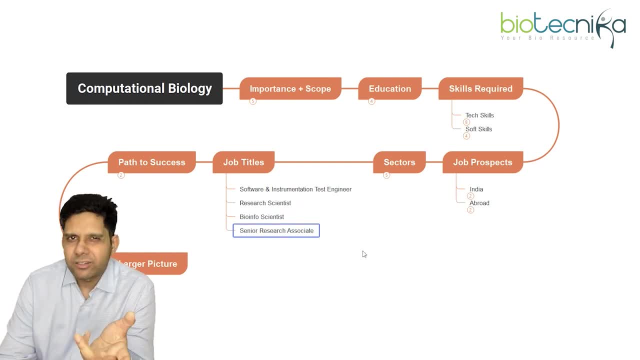 called research scientist or a bioinformatics scientist or a senior researchers associate, depending on you know, principal scientists, all such things will be there, depending on the company and the ladder. but yeah, these are the job titles you can expect, but this is not a complete list. this is just a reference list. 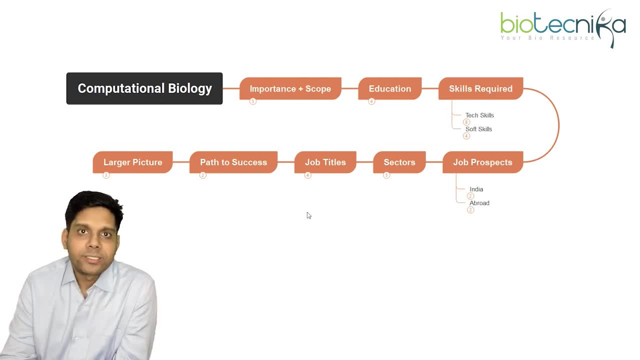 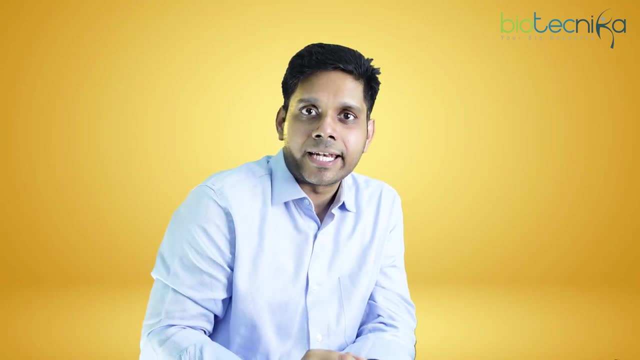 which i'm giving you now, the very important thing which you all should know is a path to success. we all want success, right? we all want to know which way i should go so that i can succeed. so you see, computational biology is a growing field. it's an upcoming. 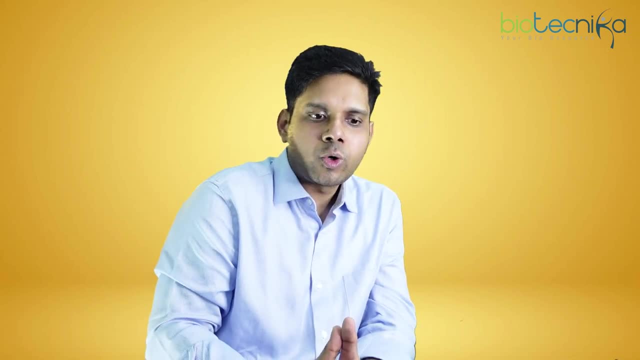 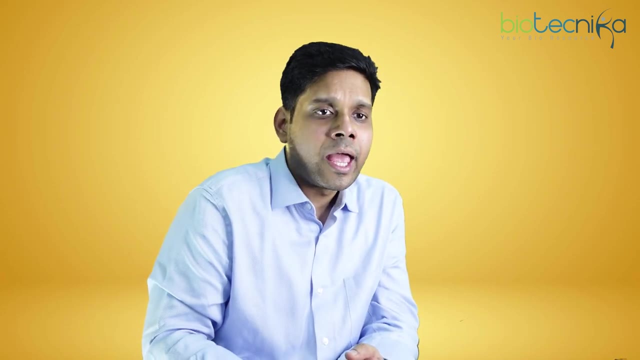 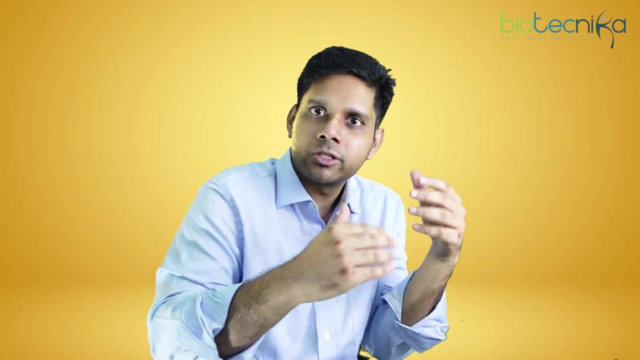 field and a lot of things are changing every day, okay, so you can't just say that, okay, i have read this book and i'm done here. okay, you need to keep upskilling yourself, okay, which is a lifelong process, and you have to know this, that you know. sky is the limit here, because computers are. 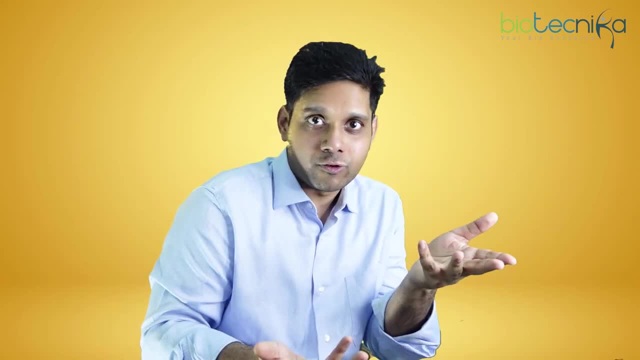 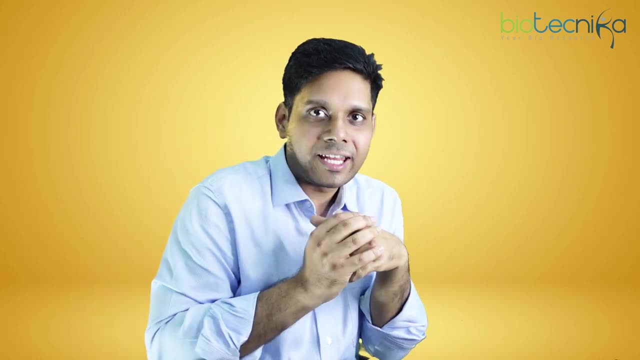 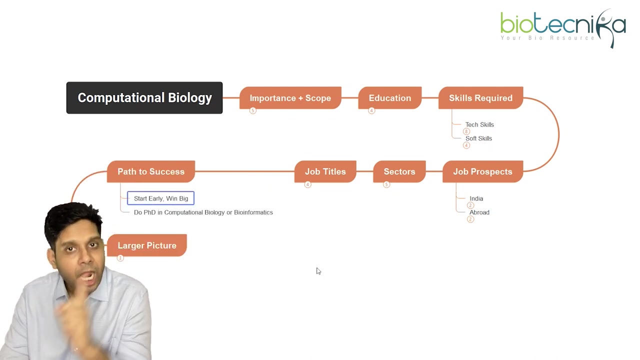 evolving and at the same time biological research is also evolving, okay. so the path is very clear here. if you are just a bachelor's or master's, you cannot go to a very high level, but if you are a phd, definitely you can quickly. this is what i have written written over here. start early win. 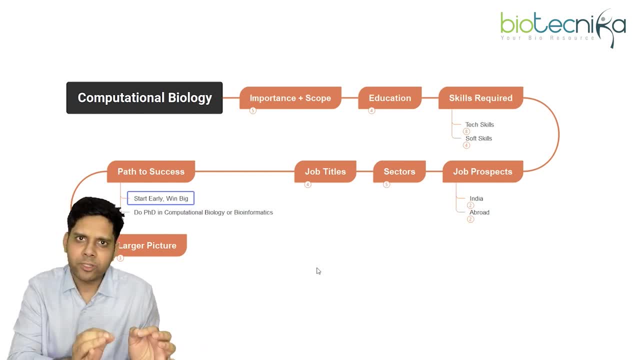 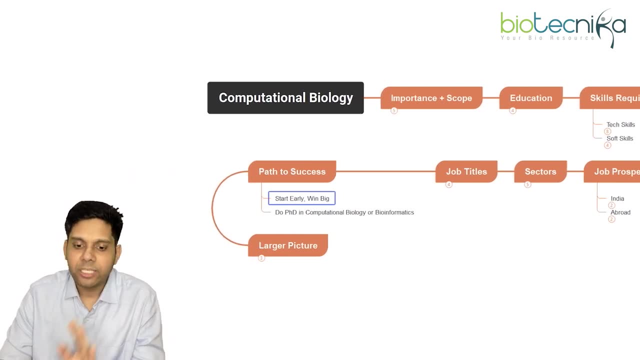 big. so if, whether you are in bachelor's or master's, wherever you're standing, start, you know, learning these skill sets, which is going to help you. okay, so, start early, win big. the next is do phd in computational biology or bioinformatics, because that will help you in your future. okay, so if you are just a bachelor's or master's, you cannot go to a. 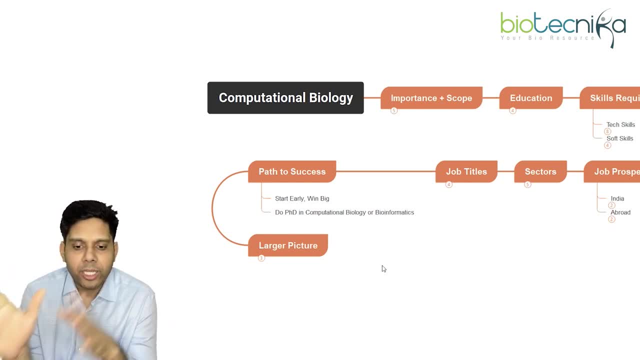 phd in computational biology or bioinformatics, because that will help you here completely okay, without a doubt. so this is a clear path to success. at early is, start learning these softwares and by the time you have cleared your csa on it or you have enrolled into phd, you will be all thorough. 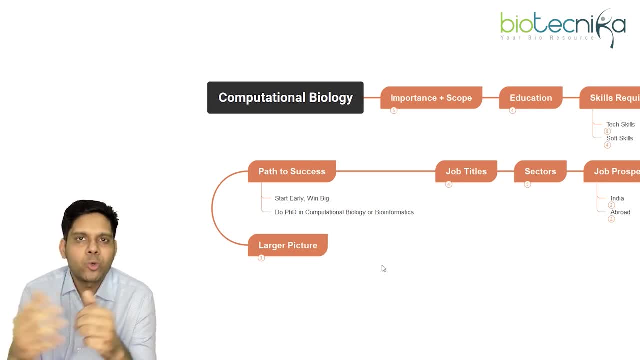 with all those tools and now you have to just apply and implement. probably you can be at this. you know, forefront of cutting edge technology called computational biology. but what if i tell you that we need to know the larger picture first? you know, when i was in my bachelor's the first day. 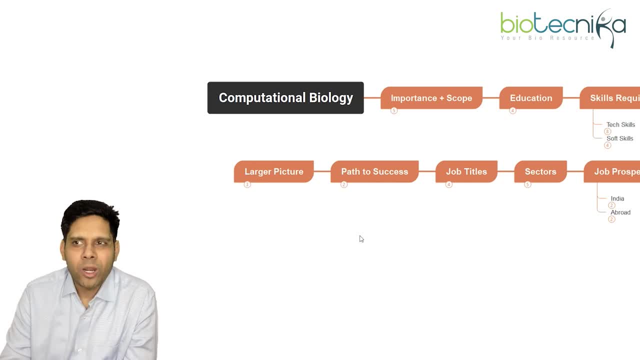 of the class, i turned back and i was like, oh my god, i have to go to a phd in computational biology. and i asked my classmate, hey, what i'm going gonna do with this course? right, because that's something which is very important. if you don't know the larger picture, we cannot have the confidence. 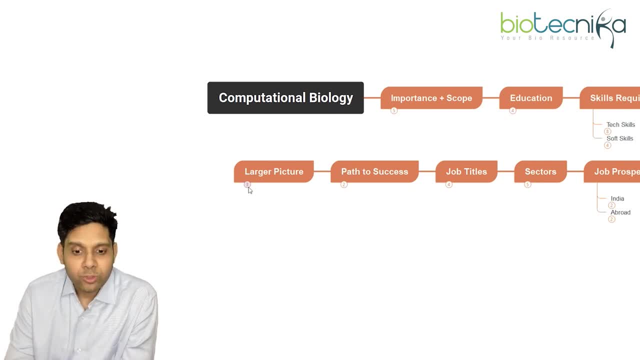 to go into that field right. so now let's know the larger picture. so the larger picture is: quantum computing is coming. in the next 10 years you will see quantum computing everywhere. quantum biology will be the next leap of computational biology and that is where, like you can see, cpus of today are much faster than the cpu of the future. so you can see that. 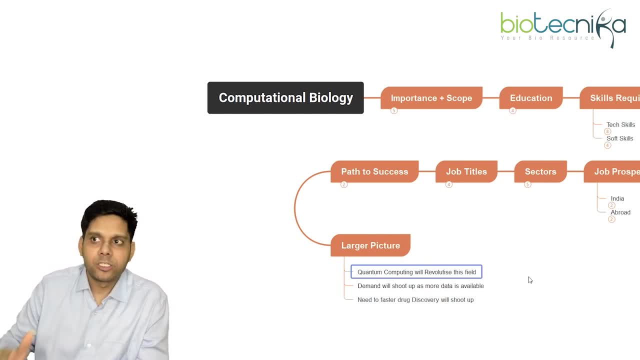 the cpus of 1990. the same way, the cpus of the quantum computing cpus of 2030 will be much faster than like 100 000 times faster than what we have today. so that is where the drug discovery process, the molecular modeling process- uh, the molecular inter modeling interaction process, all this will 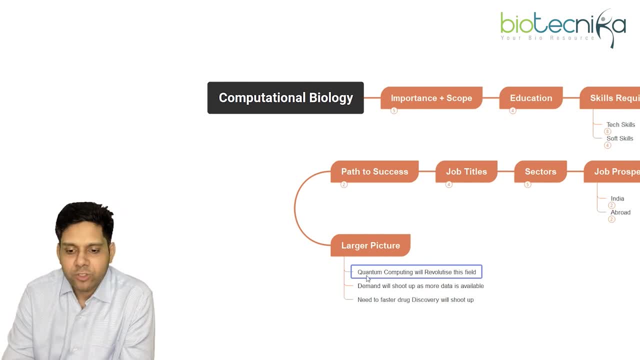 get accelerated, so that's where you can take advantage of this ever-growing field. the next one is the demand is going to shoot up as more and more data is getting available in epidemiology drug. all that is going to help you. and then there is always a need for faster drug discovery, because 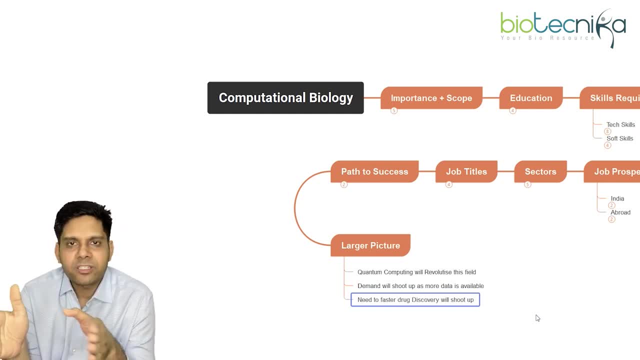 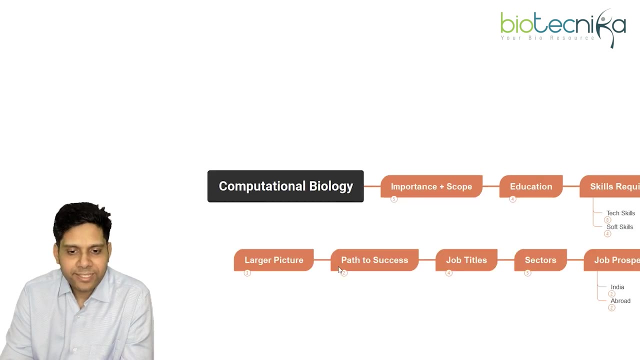 the population is exploding, the barrier between animals and humans is shrinking and that is where the- uh, you know, zoonotic diseases are jumping into the humans. so that's where, uh, we need faster drug discovery process, right? so this is, this is the larger picture we have. so more or less i have 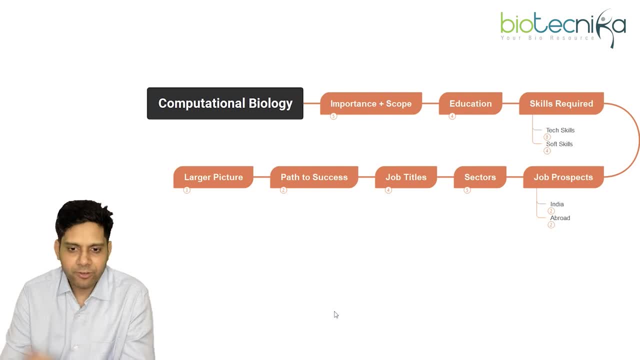 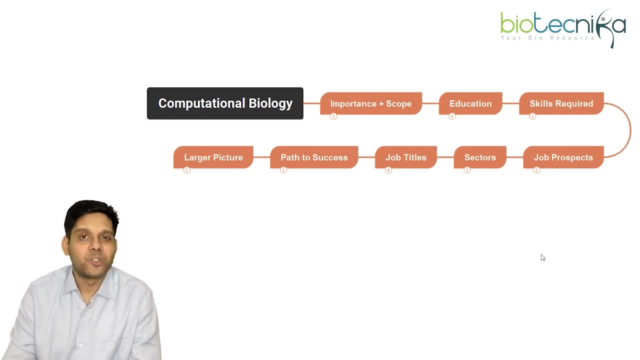 uh, given you a very thorough and clear picture, very informative uh picture here and through the help of this flow chart. but yeah, see, i can show you the direction. you have to go that way and whenever you go that way, you will have questions. so all you have to do is put those. 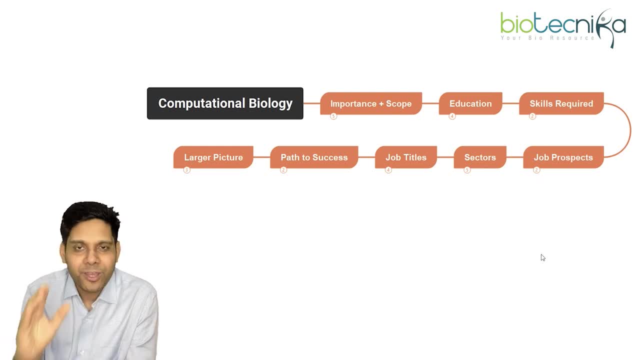 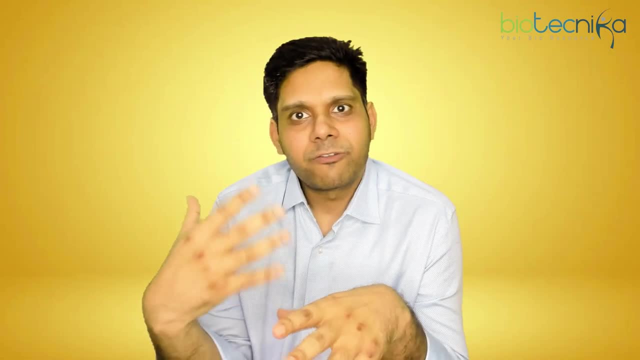 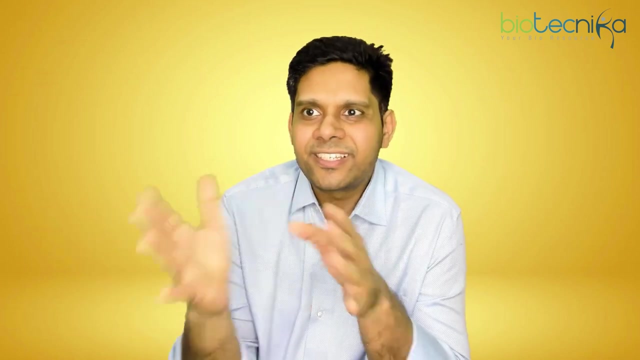 questions down in the comment section. i'll try my best to answer all of you as fast as possible, but in the meantime, remember this computational biology is growing. a field is going to grow thousand times from today, or ten thousand times from today, but it is just like if i had told you. 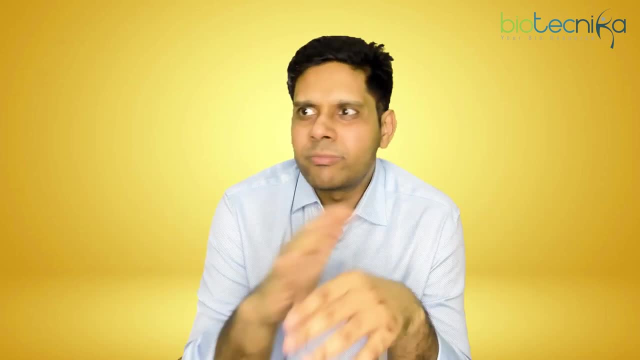 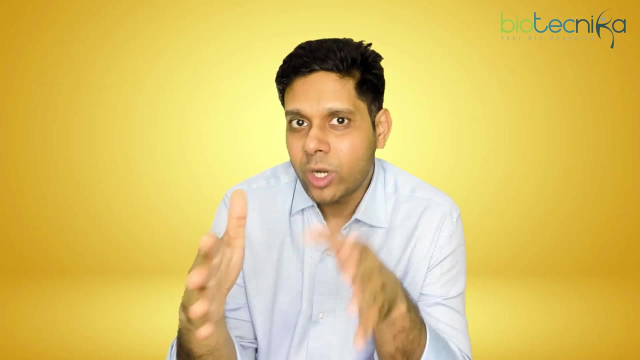 to invest in infosys in 1990 when it started, and you would be, you'd be like no, i don't think this company is ever going to grow. and today you can see, infosys is a, you know, 100 billion dollar company. so what i am trying to mean to say, i mean to say here, is, when you start early, invest in the right. 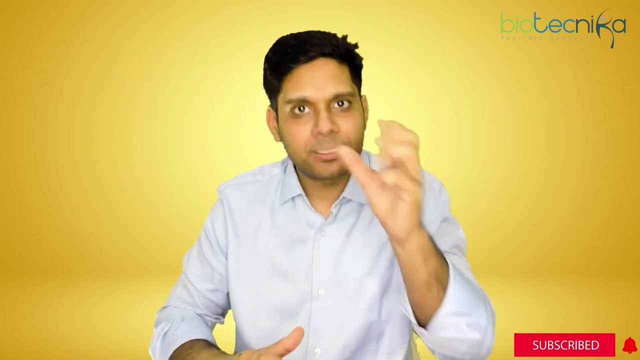 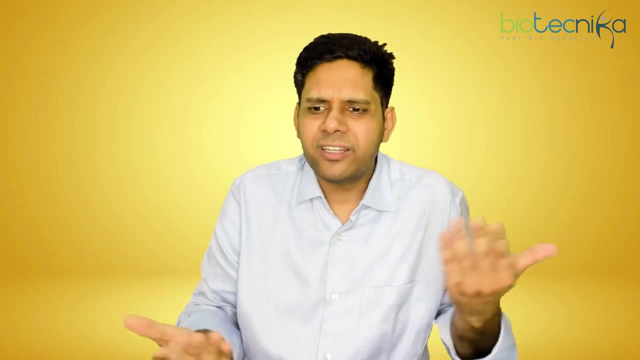 field. you are going to enjoy the speed. you are sitting on the shoulder of computers and evolving biology. you grow faster compared to anyone else and it doesn't harm. you know, the skill sets which i just showed you, the skillsets which i just showed you, the skillsets which i just showed you, the skillsets. 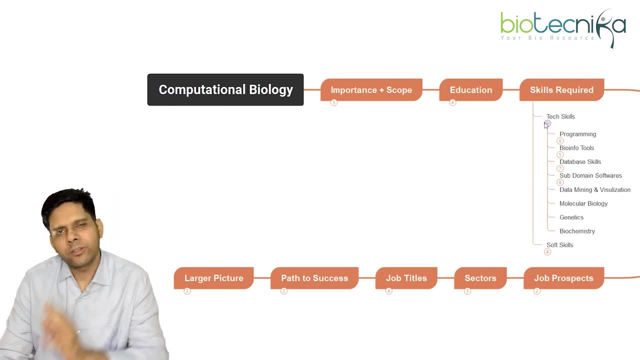 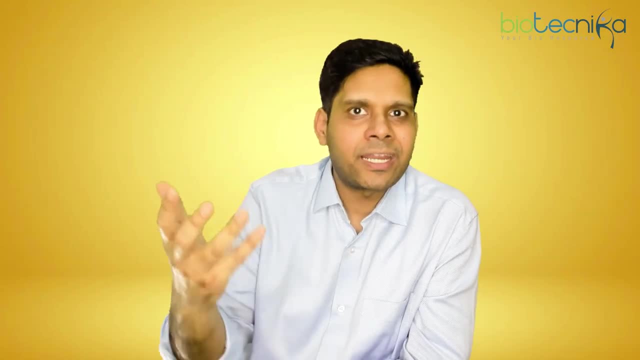 you here. like you know the technical skills, it won't harm you whether you were in any research. these things will come handy. okay, and the best part: when you start early, your understanding develops and once you have the understanding it is better to evolve. you know, do research because 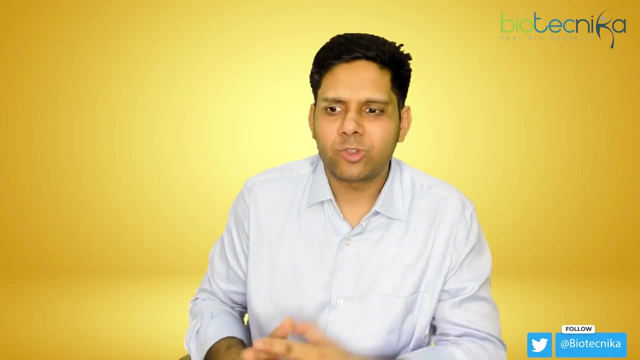 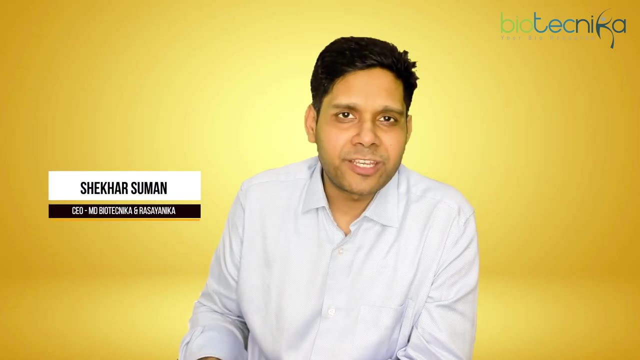 you would already know things which people are still studying okay. so i personally feel, if i was you, i would have jumped into this field. this is amazing field. so this is all about today's video. thank you so much for watching and i'll see you around in the next video. till then, please take. care and bye.